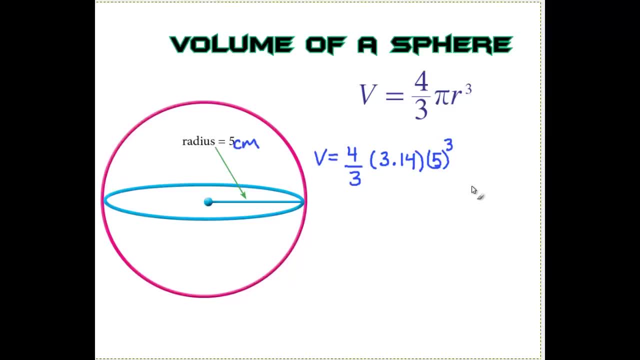 we followed our formula and we're going to round our answer to the nearest hundredth. When working with these formulas, sometimes, and with some of these numbers, when we start doing our calculations they're going to be long, maybe large, non terminating decimals. they might go on forever. so we're just gonna round to. 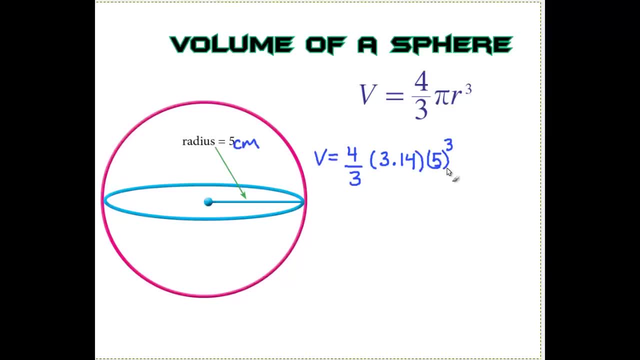 the nearest hundreds place. so let's go ahead and get started. we know that this here expanded out. 5 to the third power is really like 5 times 5 times 5. don't make that mistake of doing 5 times 3 like a lot of students. okay, and then we 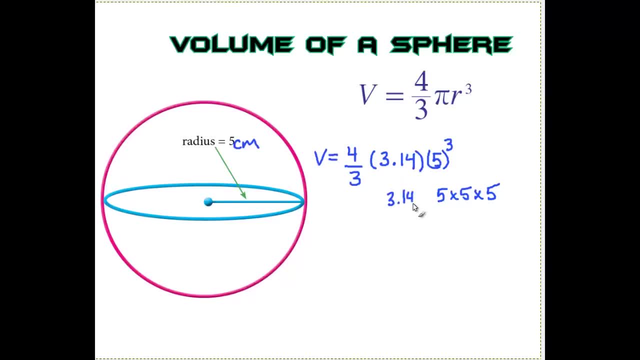 have our 3.14 for pi and we have our 4 thirds that we're gonna multiply by. so let's start with our easy stuff over here. we know that 5 times 5 is 25. then 25 times 5 gives us 125. then we bring down what we have left and we'll just 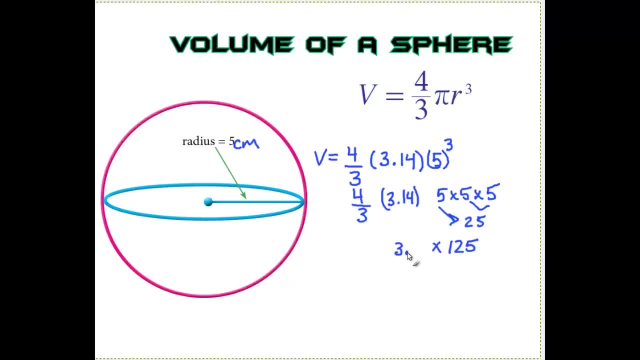 take these parentheses out. we have times three, point one, four. okay, so we're gonna do the same thing again. so we're gonna do the same thing over here, Whether it's in parenthesis or the time sign. we know that this means multiplication, and then we're also going to have to multiply by this 4 over 3.. 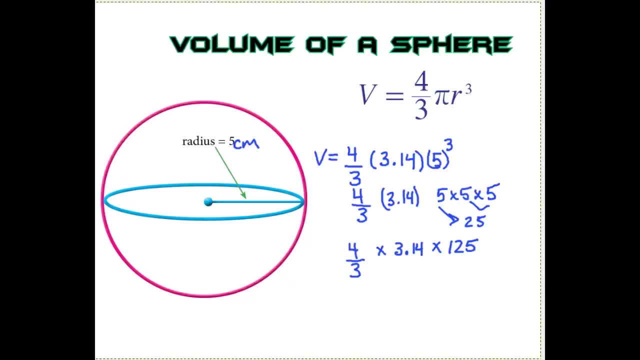 Okay, so let's go ahead and multiply 3.14 times 125, and that gives us 392 and 5 tenths. Now we just have to multiply by our 4 thirds, And this is probably the trickiest part for students. 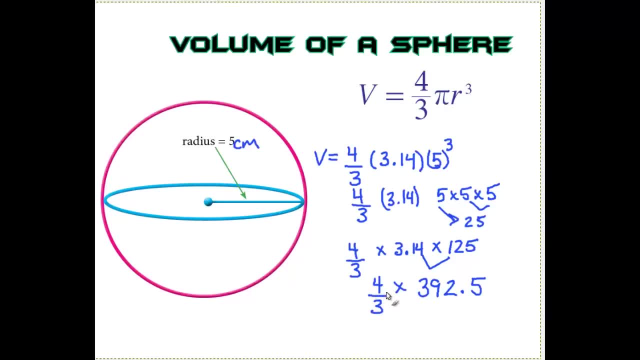 but an easier way to do this is to know that we're going to have to multiply 4 across the top and then divide by 3 on the bottom. So let's go ahead and let's do our multiplication of 392.5 times 4.. 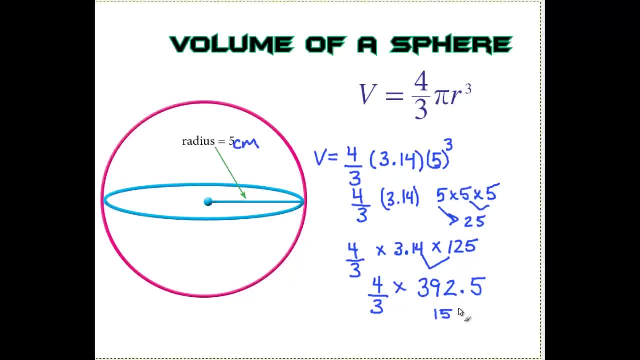 That gives us a nice 1,570.. And our last step is we're going to bring that 3 down here and divide by 3.. So our volume After we do our division here is v is equal to 523.33..